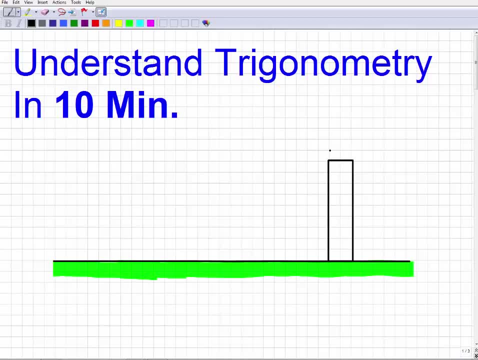 Now, how could you go about doing that? Now, it would be pretty difficult, right for you to stand up here and drop a tape measure all the way down to the bottom. I mean, yeah, there's probably all kinds of different ways you could devise. you know, maybe drop a rope all the way down there, then bring it to the ground and measure it out. 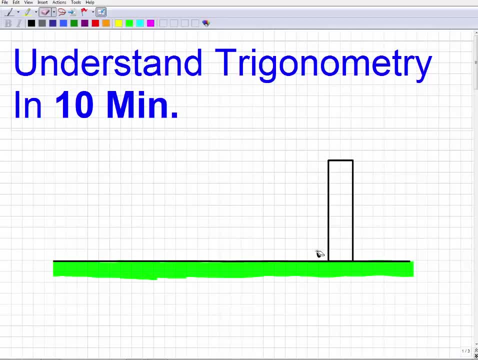 So you could somehow wrangle your way to get the height of that building. But let's suppose you couldn't even get to the top of that building. Okay, let's suppose. well, what if I told you: you know, find the height of that building, but you can't get to the top of it? 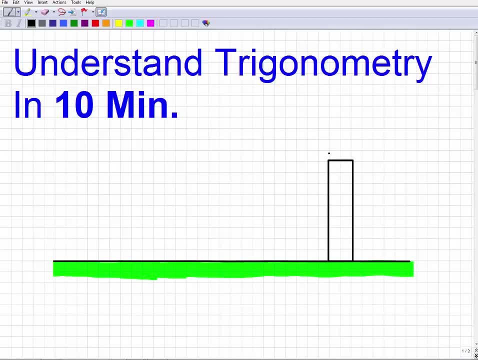 In other words, then you're going to be like: well, okay, well, how do I do that? Well, then you're going to maybe try to estimate it, But with trigonometry you can get the precise, exact height, and this is the kind of problem that trigonometry allows us to solve. 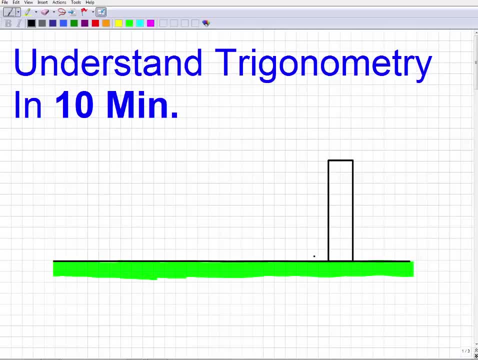 So how do we do that? Well, I'm going to kind of show you the basics of what we would do here, and then I'm going to get into actual instruction here in a second. So, with trigonometry, what it allows us to do to solve this type of problem is the following: 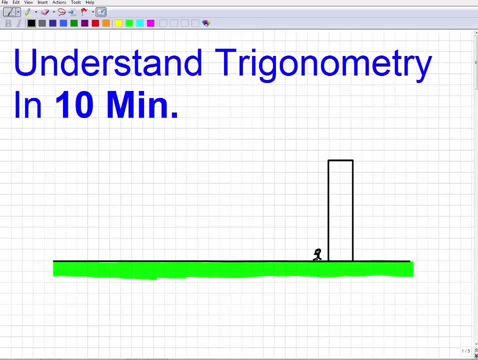 Let's say, you were down here at the bottom of this building and you said, okay, what I'm going to do is I'm going to measure, I'm going to go out a certain period. I'm going to say, let's say I'm going to go here. 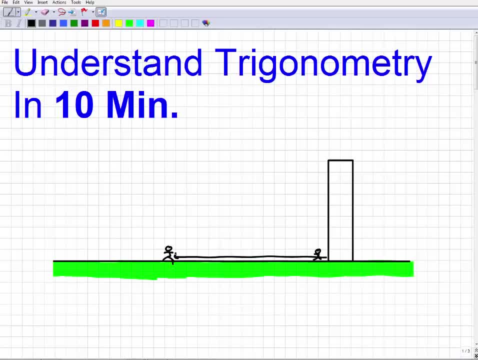 All right, and call that distance whatever you want, Let's call it. oh, let's say we went out 300 feet. Okay, we went out to 300 feet, And then at that point, you determine the angle up to the top of the building as you see it with relation to the ground. okay, 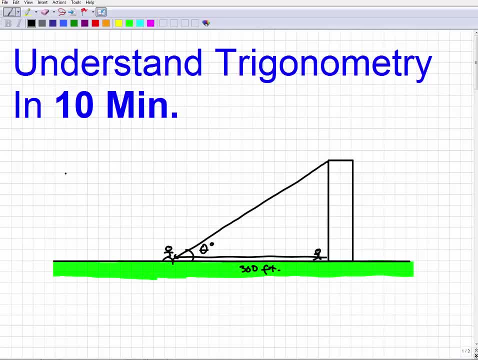 So how could you do that? Well, there's basic instruments. You can get a protractor, If you remember what those things are. it's like a little ruler down here that has like 0 degrees, 180 degrees, and you just kind of measure different angles etc. 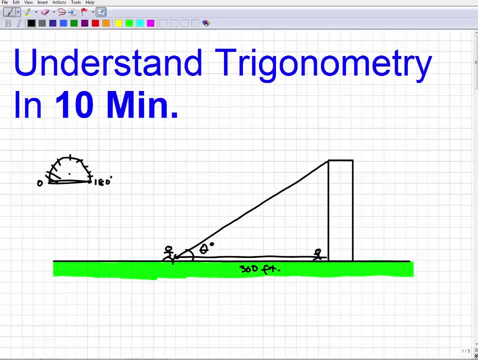 You can kind of flip this thing upside down and dangle a string. There's all kinds of little ways and not terribly sophisticated ways, to get a pretty good sense of what that angle is. Now, of course there's other instruments that would give you the precise angle. but let's say, even you kind of like eyeballed it out and you kind of did whatever sketched out. 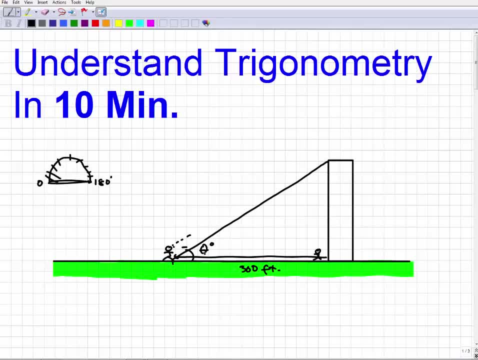 Anyway, they're kind of getting off on a tangent here. but let's suppose you were able to determine that angle. Well, as long as you knew the distance from here to here, this distance away from the building, let's say it's 300 feet again and you got this angle. 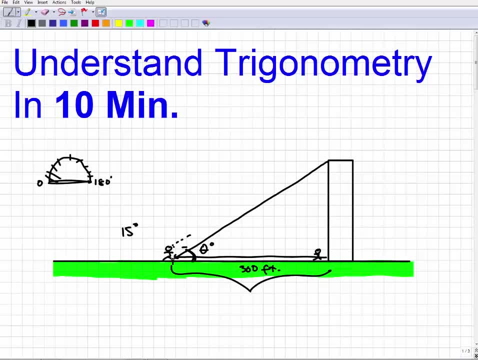 Let's suppose in this example it's 15 degrees. You're seeing the top of the building up here from where you're at to the very bottom of the ground. You're seeing that at about 15 degrees above the ground, like so. 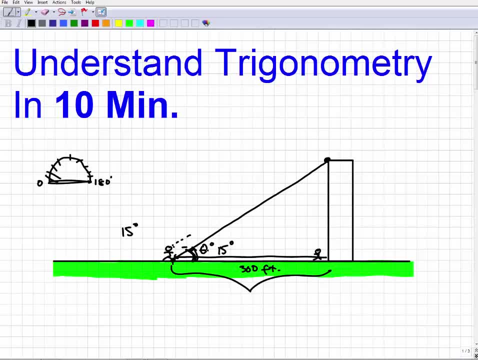 With those two pieces of information and, of course, trigonometry, you can determine the height of the building. So that should be pretty cool. I mean, that's a pretty big problem, right to measure the height of the building without being able to go to the top of it. 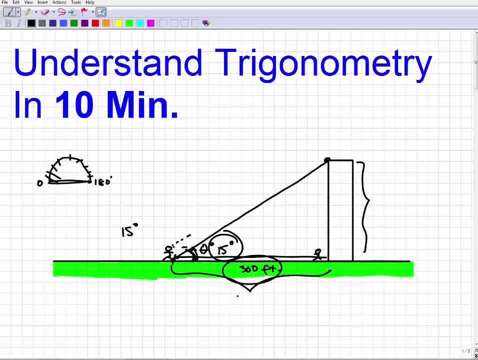 So for you just to have these two pieces of information and to be able to get the precise height of the building is very, very powerful. Now, not only can you get the height of the building, you could also get this distance as well. 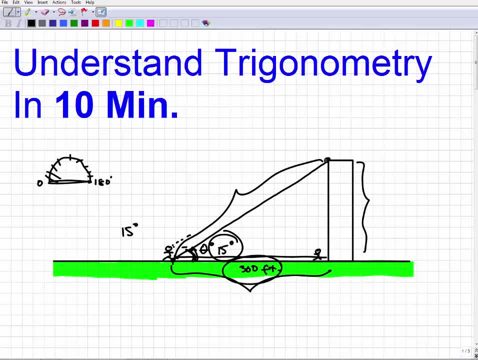 Let's suppose you wanted to string a wire or something, for whatever reason, from the top of the building down to where you are. You get the precise distance using trigonometry and another thing in mathematics called the Pythagorean theorem. Don't want to get too far ahead of myself, but it's not that difficult. 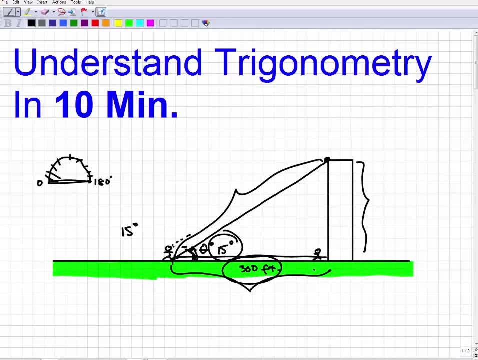 Once again, these big concepts- trigonometry, calculus- yeah, there's a lot to learn and there is some complicated aspects to them, But the essence of what they are is not overly complex and they're very beautiful in a lot of ways, because think about it. 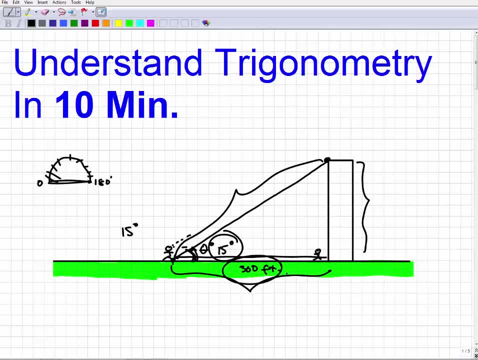 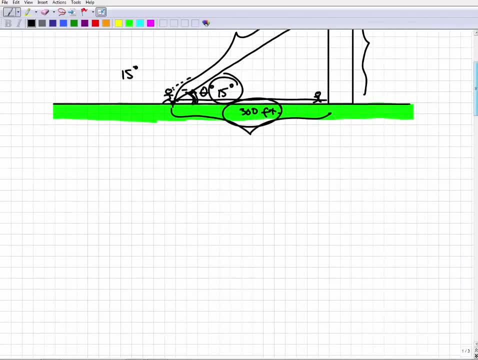 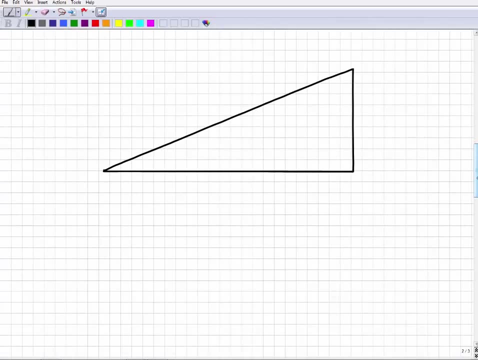 I mean, with some mathematics you can solve this problem, and we're going to solve that right now and it's not going to be that difficult, So let's go ahead and do that. So what we want to do is we want to break down our problem into a triangle. 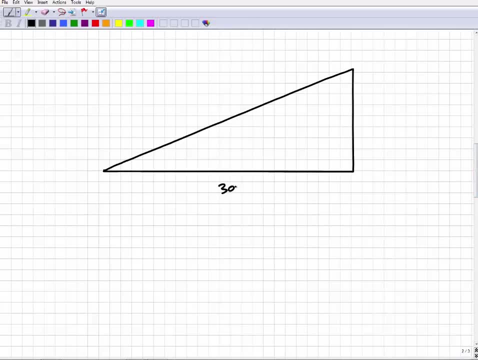 So let's suppose this is the ground, Let's say this is 300 feet and this angle here, let's say, was 15 degrees, and this would be like the top of a building up here, Top of the building, and then this is obviously the ground level. okay, 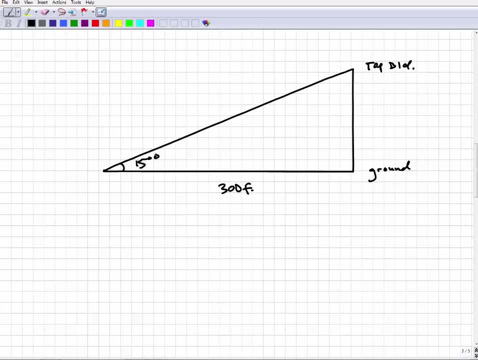 Now there's a couple things here. Let me write that a little bit better. There's a couple things here that we have to be aware of in trigonometry, So you can see how I kind of made my depiction of my scenario here using a triangle. 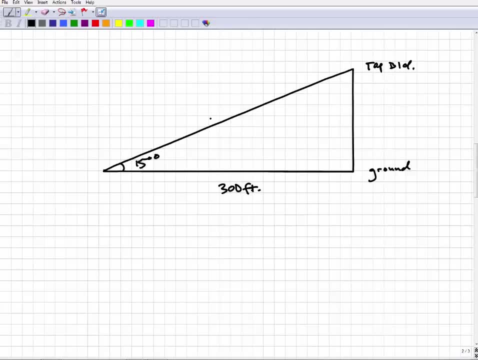 Well, in trigonometry we use triangles to kind of depict what's going on, but not any triangle. We have to specifically use triangles. We use a right triangle. okay, Now, a right triangle we denote with this little symbol here: 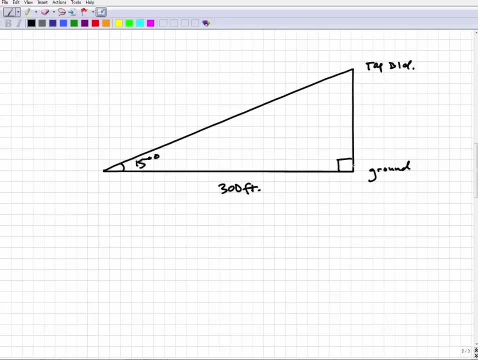 It's a little box in the corner of this right angle, okay. So if you don't know what that means, a right angle is a triangle that has a 90-degree corner in it. okay, And we denote that this way. We don't write 90 degrees. 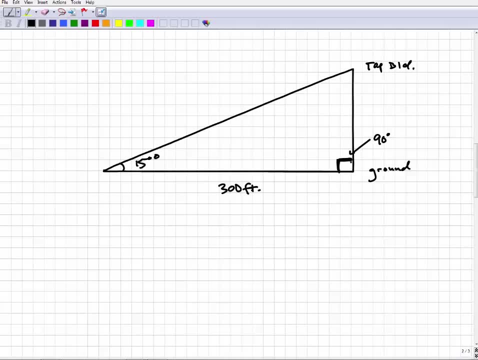 We put this little square symbol, okay. So if you see a triangle like that, that means it's right. This is 90 degrees. What we study in trigonometry, or the mechanics of it, requires us to use right triangles. Now there are other techniques that we use with non-right triangles, but that's more advanced, okay. 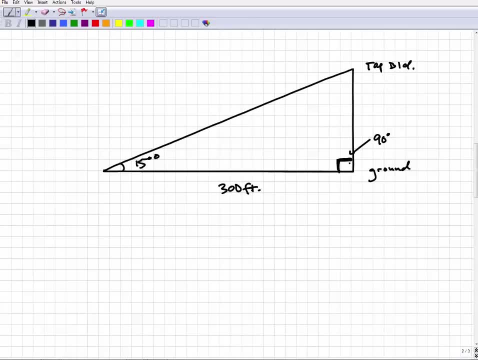 So the fundamentals of trigonometry are going to be based upon these right triangles. Okay, so I'm going to get rid of this. So we're looking for this distance here, right, We're looking for this distance, And I said to you that if I gave you the degrees and the distance away here, we can get this distance and we can. 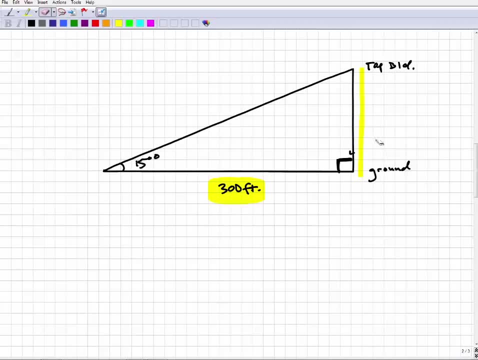 So this is where we're going to learn about trigonometry, okay, So let's just keep this in mind. This is our kind of representation of the problem, And now let's get into the core, fundamental concepts of trigonometry. Okay, so trigonometry is based upon the following: okay, 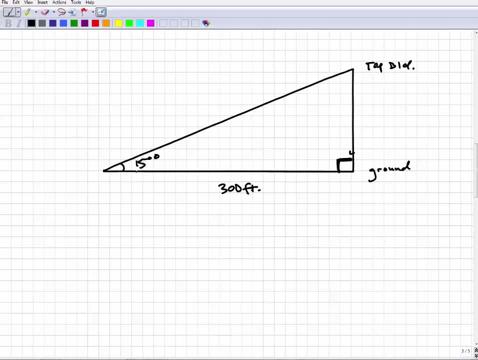 We have an angle. all right, Now, in a triangle we can have three angles. We can have this angle here, this angle here. Let me draw it this way: We can have this angle here, this angle here, or this angle here. 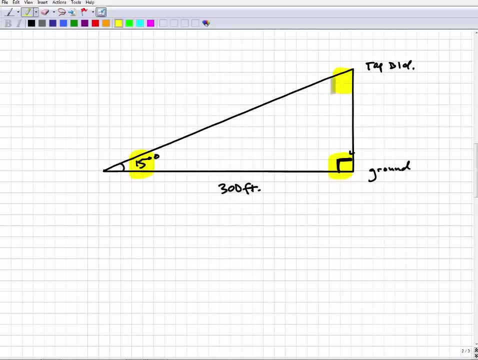 Of course, we know this is 90 degrees, but these are going to be other angles. okay, Now, in this triangle we also have sides. okay, So we have this side or this distance to this triangle, this side here and this side here. 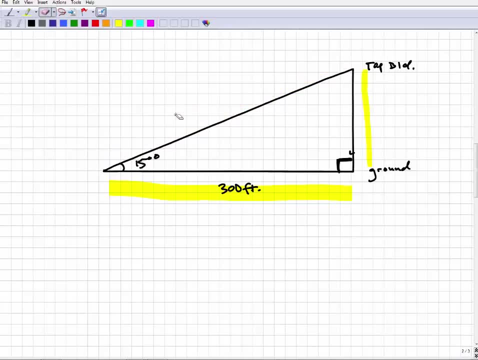 So what we're going to have to do is we're going to have to give these sides and angles kind of names. okay, Now, this angle right here in this particular corner. we're going to learn these names here in a second, So let's start with this angle. 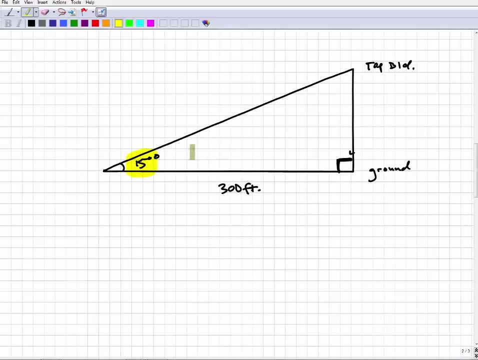 Now, relative to this angle, the side of the triangle that's far off, okay, Away from it. this side here we have a certain name to it. Then we have a name to the side of the angle that's right next to it, okay, 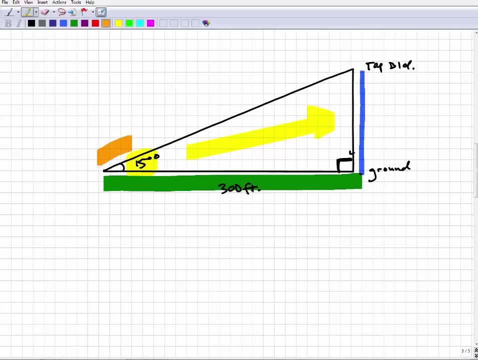 And then there's another name to the longest side of the triangle. Now, each triangle, no matter what you have, you can clearly see which side is the longest. That's this side. okay, Now this side here is the side of the triangle that's next to the angle. 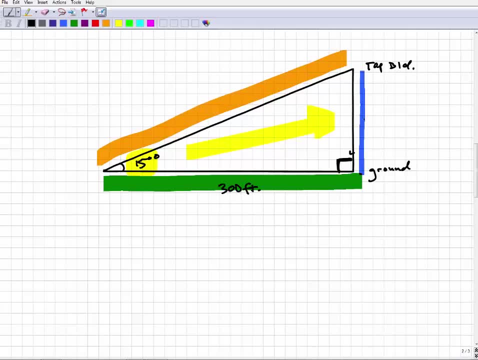 And then we have this side, And then we have a side that's away from the angle. okay, So let's talk about what these sides are respective to this angle. So the first side is called the opposite side, So we're just going to put an O, okay? 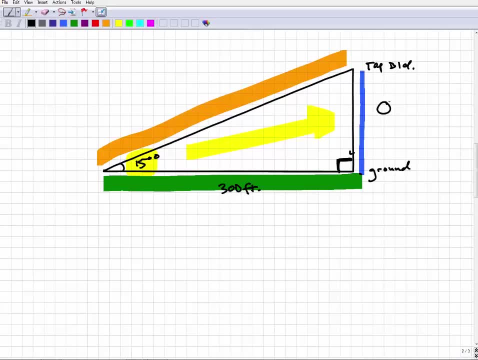 This is the O opposite of this angle, far away from it. okay, Now the side that's right next to it. okay, there's a word for that That's called adjacent. This is actually called the adjacent side, okay. 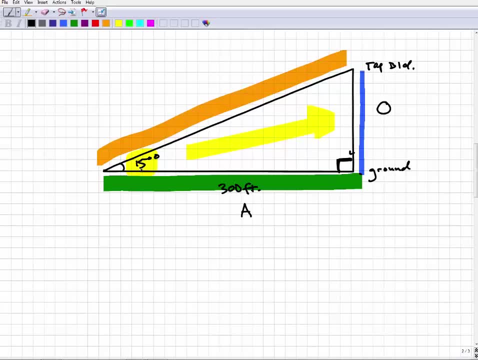 This side is the side of the triangle that is forming that angle. You follow, You see what I'm saying. This side here actually connects with that angle, It's forming it. That's called the adjacent side. Again, this side that's far off, okay, immediately opposite, is called the opposite side. 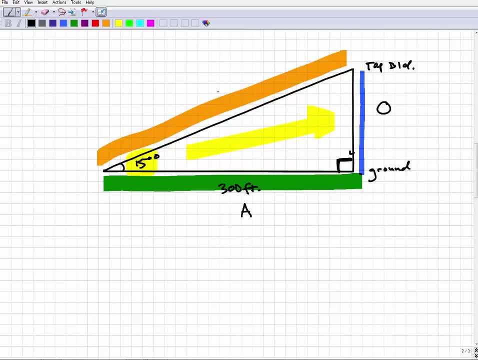 And then the longest side of a triangle is called the hypotenuse, And that's just. we represent that with an H. okay, It's hypotenuse, All right. So this side of a right triangle is called the hypotenuse. 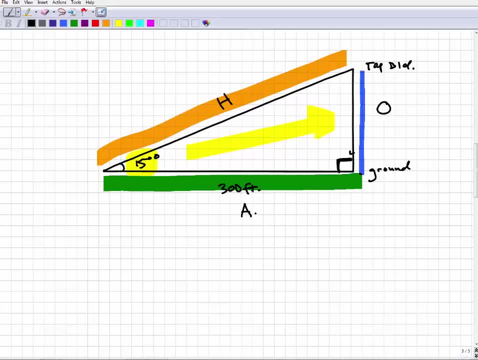 So now we have H-O-N-A. okay. Now this is where I always like to teach trigonometry. People go kind of crazy when I'm going to tell you this Trigonometry is based upon this crazy phrase: okay. 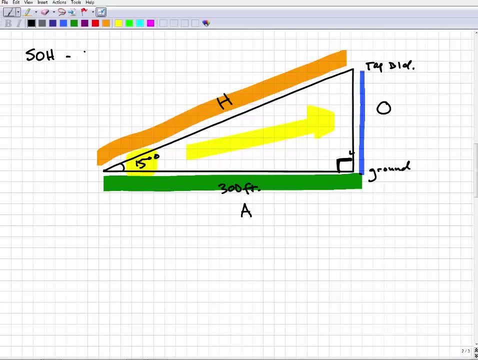 It's called SOH-CAH-TOA- SOH-CAH-TOA. It sounds kind of crazy, I know it does, But trust me, you'll remember this forever. all right, Once you learn it, you'll be like it'll be stuck in your brain. 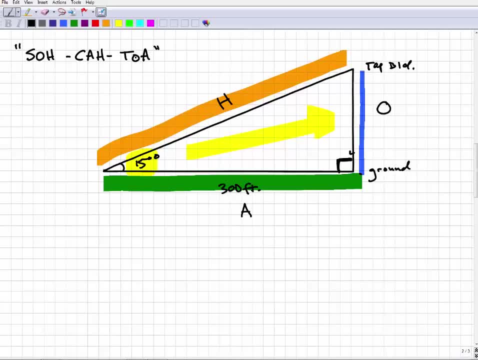 SOH-CAH-TOA. And what does that mean? okay, Well, in trigonometry we have these functions, okay, And if you look on your calculator, if you have a scientific calculator, you'll see these buttons. okay. 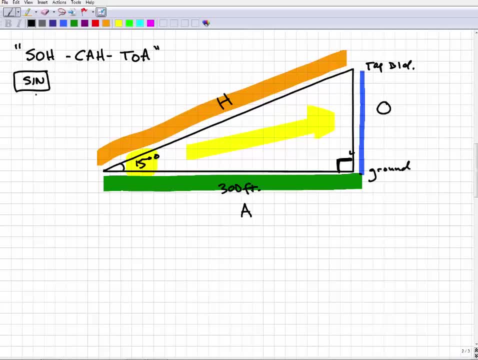 S-I-N, And it's not sin. I know it's spelled the same way. It's not like you know, you're going to church and you're committing to sin. They'll be committed to sin watching this video. Anyways, hopefully not. 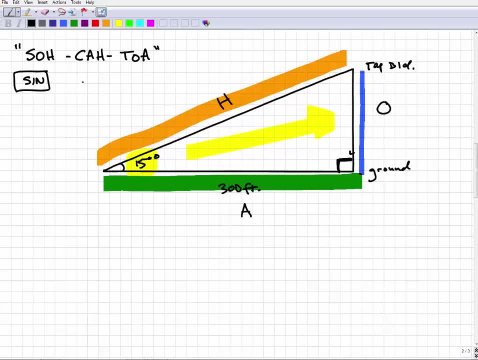 But no, this is called pronounced sine Sine. okay. The next one is C-O-S. This is pronounced cosine. all right, And this is just obviously the abbreviations, And then we have T-A-N. okay, That is the tangent, okay. 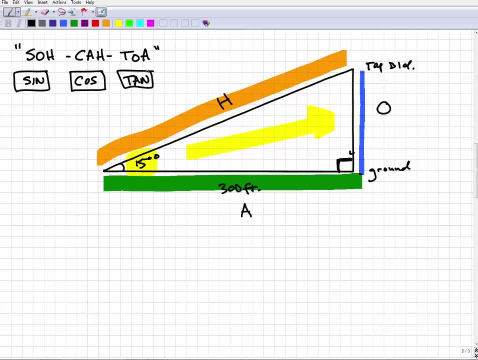 So we have sine, cosine and tangent, And these are the main things, the main functions that are going to help us solve these problems. Now you'll understand what these are here in a second. So let's talk about the sine, okay. 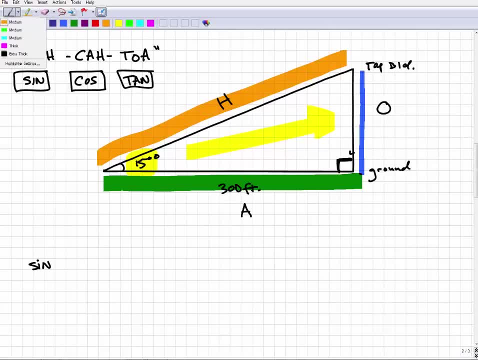 So the sine is going to be- let me actually use this color here- The sine is defined as: so When we think of so, we think of the sine. So the sine is the sine of some angle, is defined as O-H, The O-H. 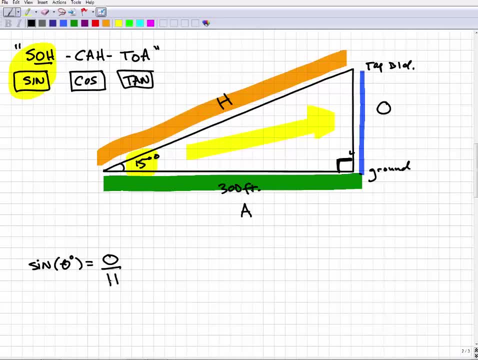 And that means the opposite over the hypotenuse. okay, So the sine of this particular angle here would be the measure of this side, the O right here, right. So if I want to get my tape measure out, or whatever, if I knew this distance and I divided it by this distance, I would have the sine. okay. 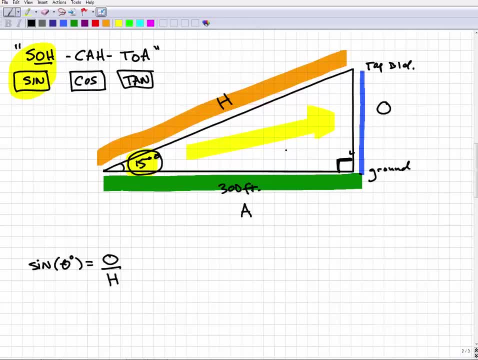 Of course we don't have those distances right now in this particular problem. But don't worry about that, Just follow what I'm saying. The sine of this angle. if I wanted to find the sine of this angle, I just divide the O, divided by the H, or we can remember that by the phrase. so okay, 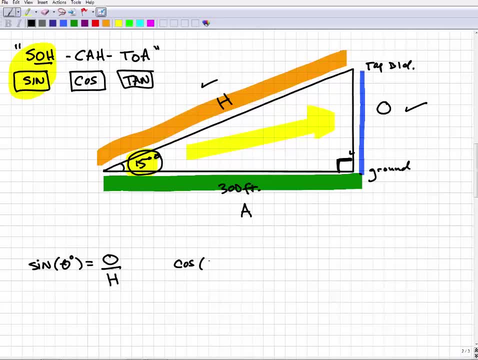 The cosine of this angle. all right, And you notice I'm just putting a generic angle here, But let's say we're talking about this one here. It's defined by k. okay, That is the adjacent over the hypotenuse. 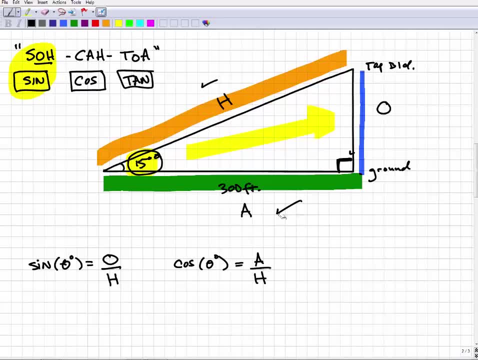 So in this case it would be this side. Let me get rid of these here. The adjacent is this side, The adjacent is this side over this side. okay, So if I divided this side, divided by that side, I would have the adjacent. I'm sorry, I would have the cosine of that angle. 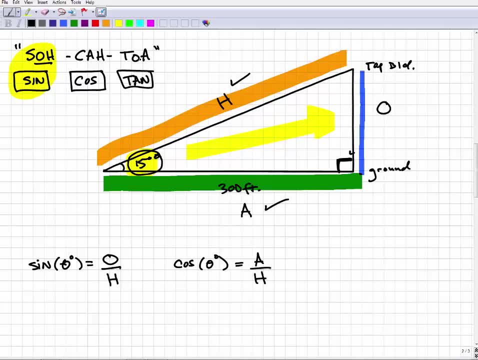 Now you could probably guess what the TOA is right. The tangent- just take a guess, if you will- is TOA. What do you think? that is O divided by H, okay, Or the opposite. I'm sorry, opposite over the adjacent. 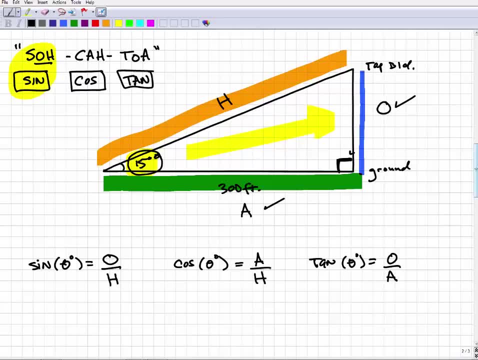 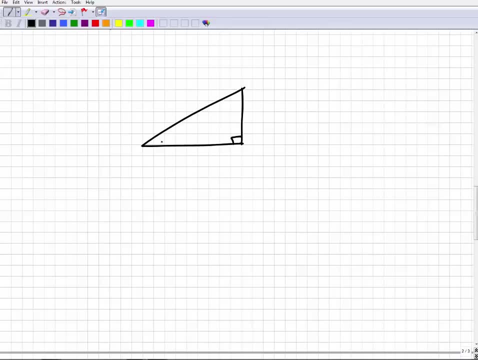 So let's take a triangle. I'm going to come back here to this figure in a second. Let's just take a real basic triangle. okay, Let's say this angle here. I don't know it. This is a 3,, 4,, 5 right triangle. 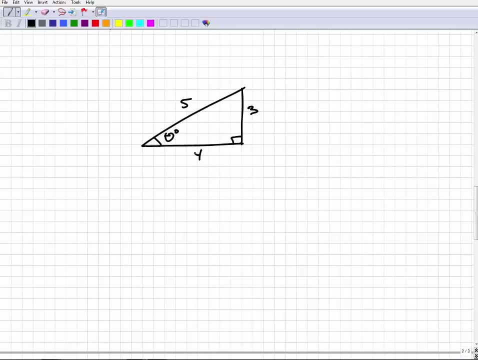 These are actual correct lengths to this particular right triangle And here's an angle here, right. So let's think about: so, okay, This is sine, So CO, right, Cosine TOA, This is tangent. okay, So the sine of this angle here, whatever angle measure this is, is going to be equivalent to what? 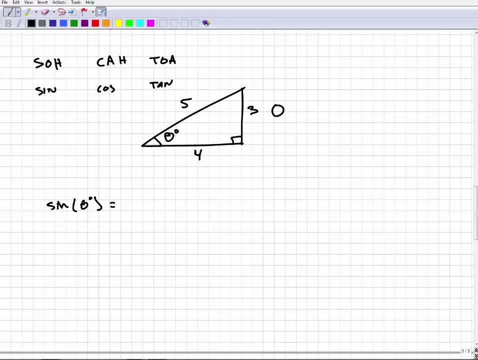 The opposite. its opposite is what? This is the opposite. whoops, This is the opposite. this is the adjacent to this angle and this is the hypotenuse. okay, So in this case, the sine of this angle here is the same number as what? 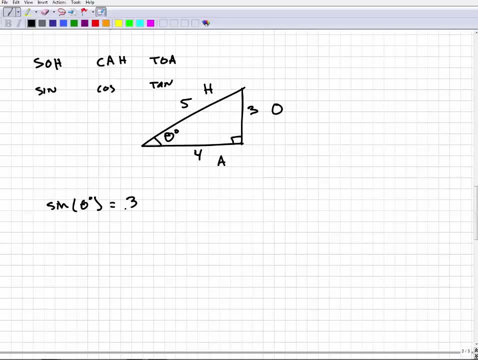 The opposite over the hypotenuse. So that would be 3 over 5, 3 fifths okay. So if we do that, if we go in our calculator and take 3 divided by 5, we're going to get a decimal of 0.6, okay. 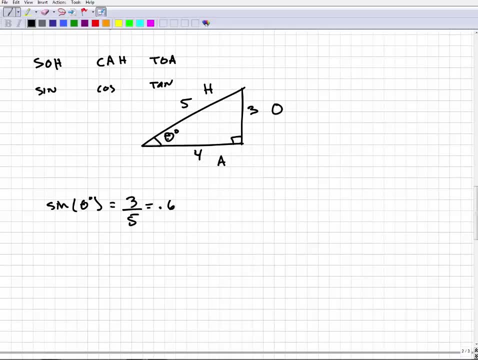 So if I knew this angle, this actual angle here, and I went into my calculator, I would know that this is the opposite. So if I knew this angle, this actual angle here, and I went into my calculator and I took the sine of this angle, okay, 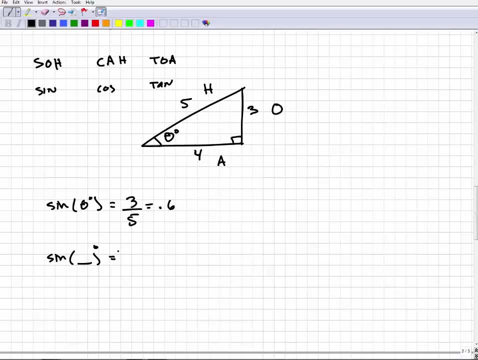 And I'm sorry I don't have this pre-worked out right now, but we'll see how this plays out in the next problem here- I would actually get 0.6, okay. So if I had this angle and I go into my calculator and I put sine of that actual angle, it would be the same as 0.6.. 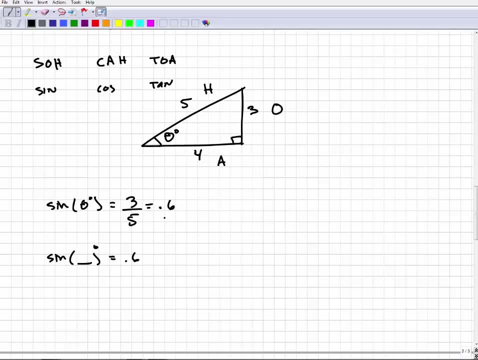 So hopefully you're kind of getting a feel for this. alright, Same thing here. cosine: Alright. So the cosine of this angle here is going to be the same as what The adjacent over the hypotenuse. The adjacent happens to be 4, and the hypotenuse happens to be 5, okay. 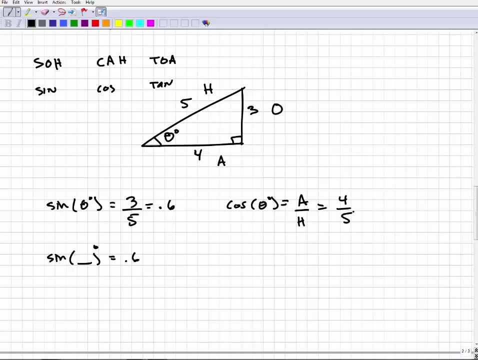 So just that decimal 4 divided by 5, 4 fifths is what? 0.8,. okay, Now you're saying to yourself: well, cosine, if I plug in, let's say cosine of 37 degrees. 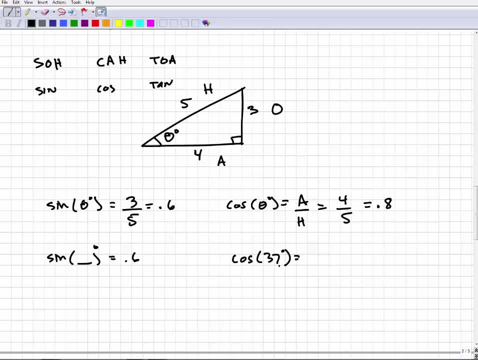 Well, how do I actually find this number? Where do you do it? Well, here's how you get that value. You need a calculator, okay, You need a scientific calculator that has its functions. Now, you don't necessarily absolutely have to have a calculator. 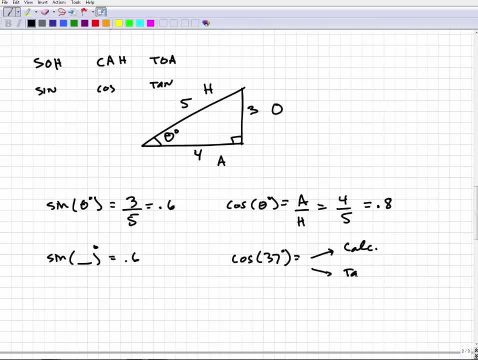 That's the smartest and best way to do it. There's also tables that us old guys, old folks used to have to use way, way back in the day, where you know you would have to actually look things up as an actual book. 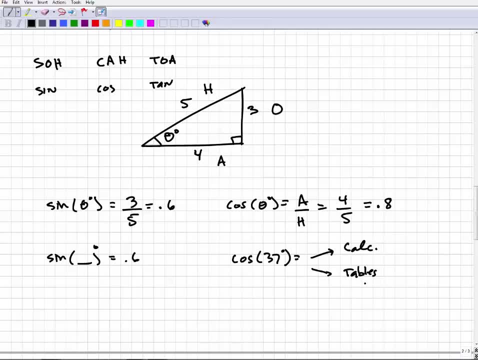 Can you imagine that in this day and age You'd actually use your textbook? You'd flip over. As a matter of fact, if you have a trigonometry textbook, you probably don't even use it. But if you go to the very, very back of it, where the table of the index is, 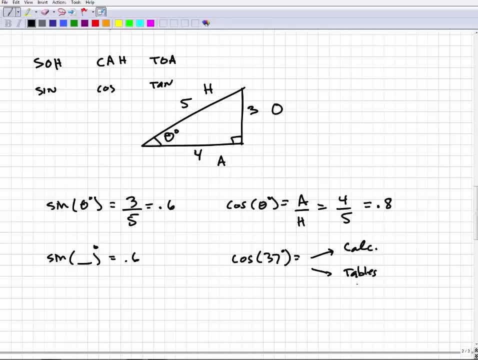 you'll see the actual tables So you can look up these values. But obviously the best way to do it is just to plug these values into your calculator. So if you go to cosine 37 and you hit enter, it'll spit out a decimal, okay. 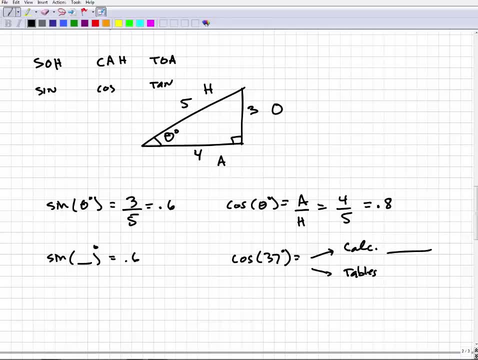 So we can get these values. but we can also get these values by just comparing these sides. So these trigonometric functions are nothing more than ratios of any two sides of the right triangle. That's all it is. So in terms of this angle here, 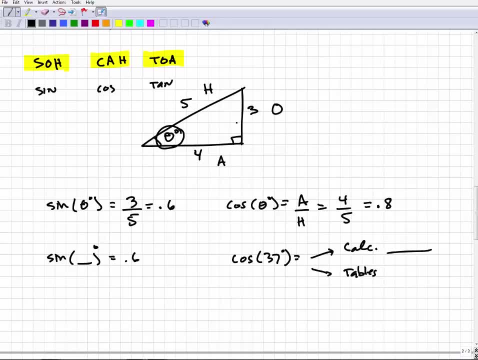 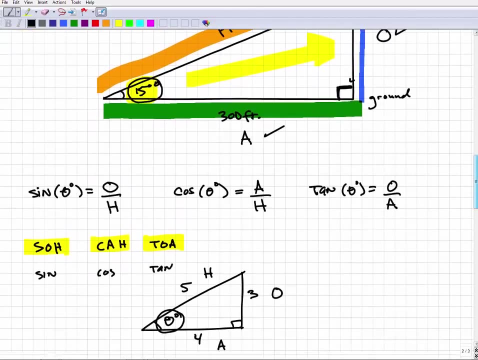 trigonometry is just basically comparing any two sides of a right triangle. It tells us information about an angle inside of that triangle. Okay, that's all it's going to do, But let's kind of pull the parts together here and see, with our problem, how this is going to work. 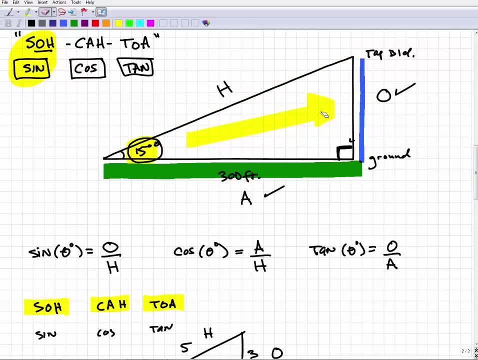 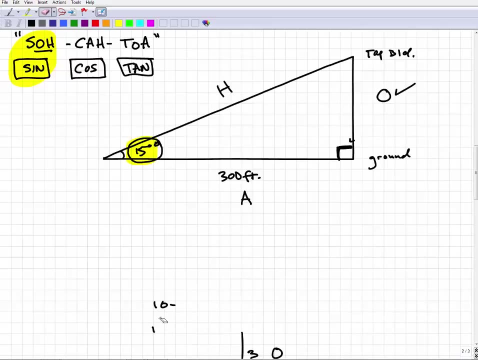 Okay, so let me erase all this and get back to our problem. Okay, so let's think about this, Remember: I want to find the height of the building. How can I find the height of the building here? Well, let's see. 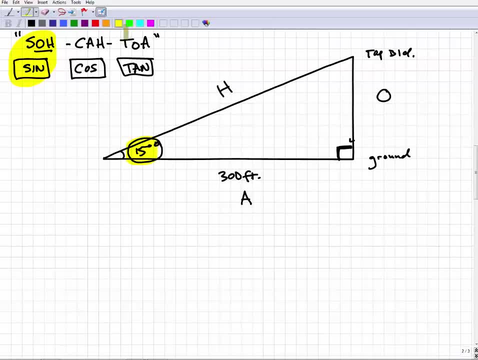 The height of the building in this particular problem. is this distance here right? So really, what I want is the O. okay, I want the O distance correct In this particular triangle. I'd like to know what the O distance is, because the O distance? 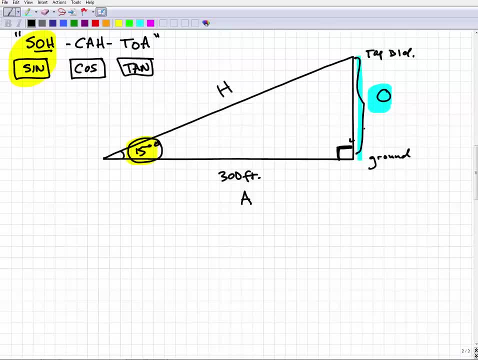 so the opposite distance here, the length, if you will, is actually representing the height of the building. But I have, in terms of my information, in my problem. I don't have the H, I have the A. okay, I have the distance of the A. 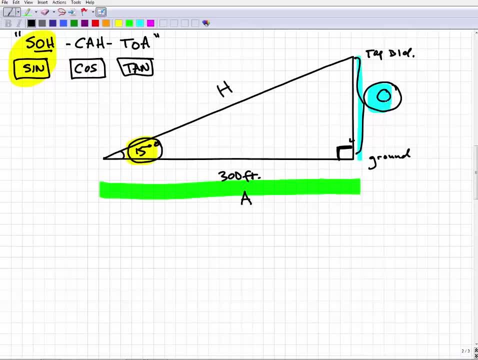 So I want O, I want the O length, but I also have A and I have the angle. So we have to think to ourselves: which of these trigonometric functions should I use? okay, or can I use Now? you could start off with one. 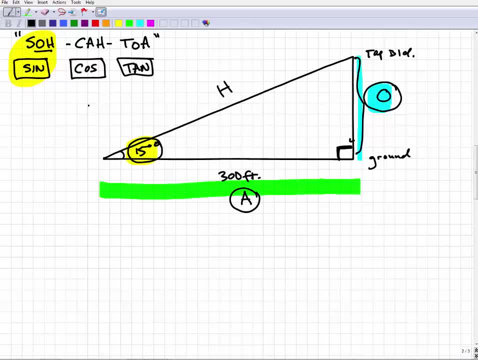 and kind of one trigonometric function may be able to get you to your answer. You're kind of using a longer route, But in this case we don't really have too many options. okay, We have to use the trigonometric function. 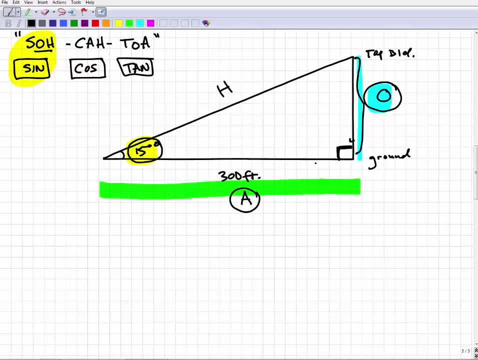 that has O and A both in it. So which one is that? So uses the OH, It uses the AH, And the TOA uses the O and A. okay, And that's what I need. So I'm going to need the tangent function here. 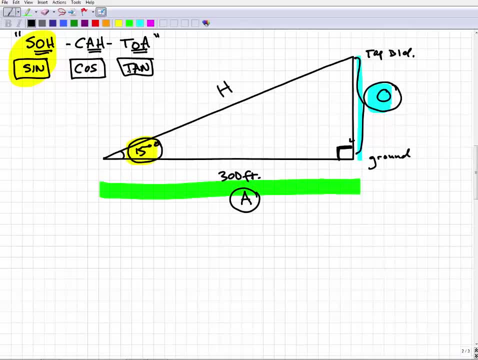 I get to select. That's what's cool about trigonometry: You select which one you need. okay, I can use the sine if I have the opposite in the hypotenuse. I use the cosine if I have the adjacent in the hypotenuse. 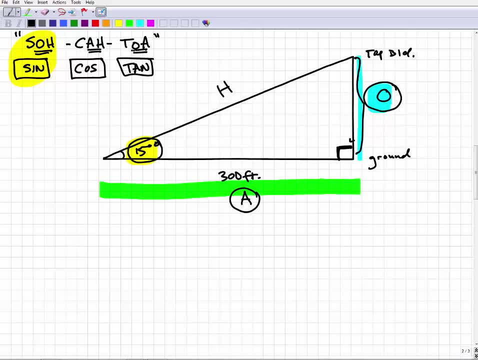 And I'm going to use the tangent if I am looking for the opposite in the adjacent. In other words, if the O and A are involved in my problem, use that Cosine. if the A and H are involved in my problem, use that. 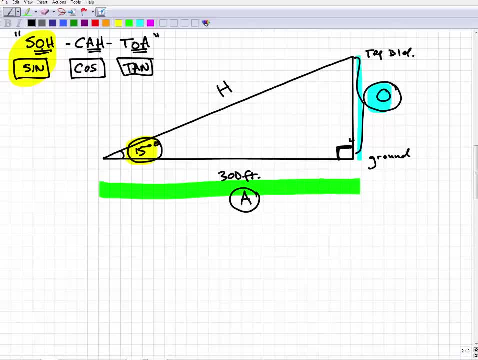 And sine. if the O and H are involved in my problem, use that. So let's go ahead and use the tangent. So how does this work? So this is going to be the tangent of this angle. Now, this angle actually is 15 degrees. 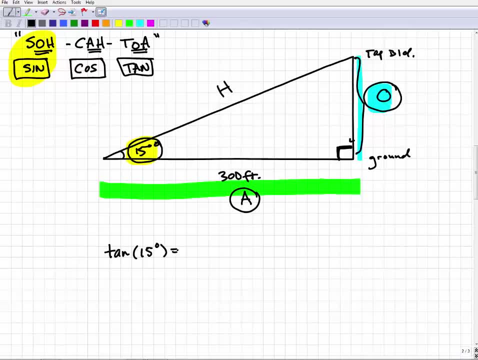 So let's plug that in The tangent of 15 degrees is the same value. Okay, now, first of all, let's go, and before I even do this, I know I'm kind of taking a little kind of few tangents- 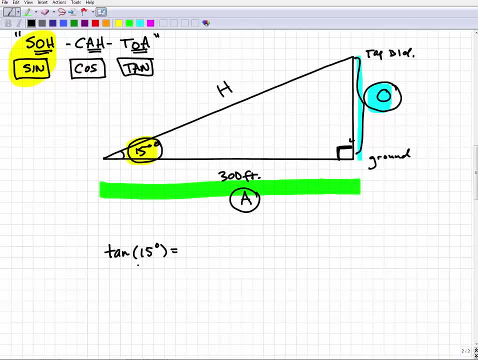 but this is important: Let's get our calculators out. And if you don't have a calculator and you're obviously on the internet, you can go. just do a quick Google search for scientific calculator and you can find out this: Okay, just take the tan T-A-N. 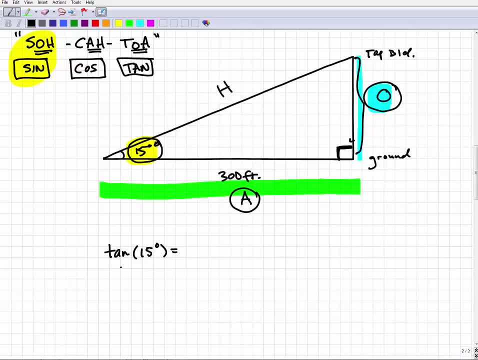 plug in 15.. So let me go ahead and do that in my calculator. We'll work together. So the tangent of 15 degrees is this decimal value of like .267.. And it keeps going. Okay, but you get the idea. 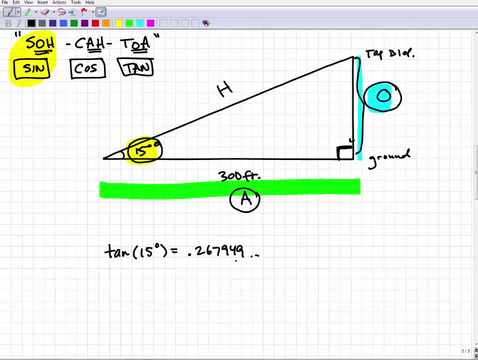 So I know what that is. So the tangent 15 degrees is this number? Okay, my calculator tells me. Of course, if you had a table of values, you can actually look that up as well, But in this problem- Okay, we have some other sides of this triangle. 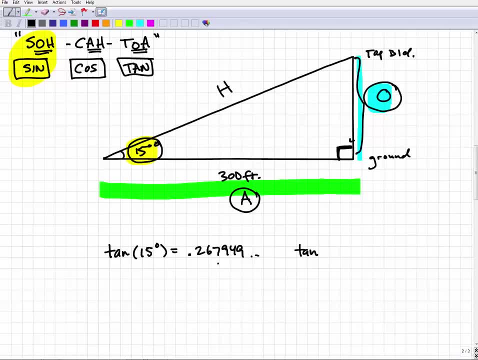 that's going to tell us the same value as well. You'll see how this works here in a second. So the tangent of 15 degrees- okay, by definition, is TOA, right, so the tangent is the same thing as the opposite over the adjacent of your right triangles information. okay, so the 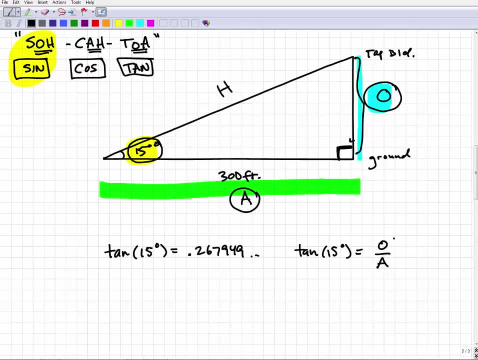 opposite. I don't know. I don't know what this is. this is what I'm looking for, so I'm going to, I'm gonna be, I'm gonna use a variable. okay, I'm just gonna say that's X. I don't know what that is, that's what I'm looking for, but I do know the. 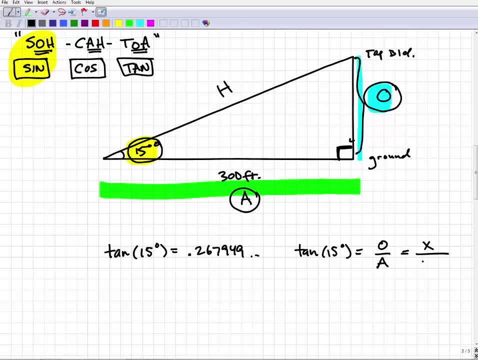 adjacent side right, the adjacent side is 300. okay, so now I have a nice little equation I have. tangent of 15 degrees is equal to X over 300, and if I solve this equation for X, I'll get my answer. so some of you are probably saying: oh how? 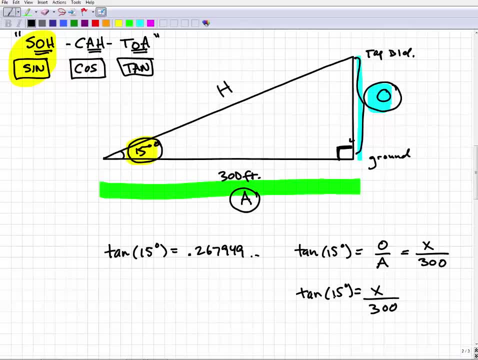 do you solve this equation? this is very complex, very simple, okay. so remember again: tangent of 15 degrees is actually just a tangent of 15 degrees. so if I solve this equation for X, I'll get my answer decimal. but I'm gonna write, I'm gonna leave it like this, okay, so tangent of 15. 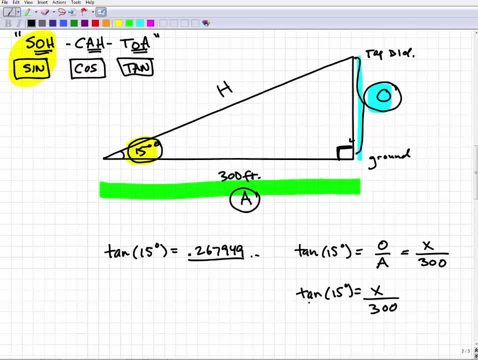 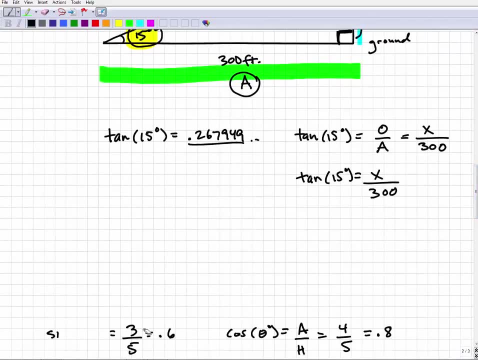 degrees is the same as this decimal point two, six, seven, etc. okay, now when we look at a problem like this in algebra- let me erase this- we always want to make a number that's compared to another fraction into another fraction. in other words, we're gonna write this over one and now I have two equal fractions: one. 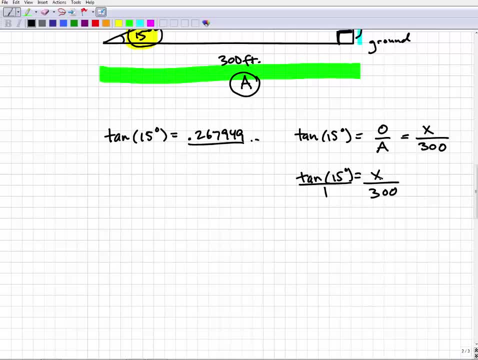 fraction equaling another fraction. so let me show you how you solve a problem like this. so let's take the fraction one half. so what's another fraction that's equal to one half? there's any number of them, right: 4, 8, 5, tenths. let's take the fraction 7 over 14. 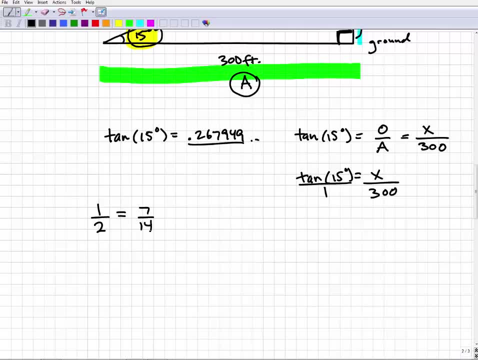 okay, now, 7 over 14 is the same thing as a fraction: 1 1⁄2. this is actually called a proportion, and the way we solve these super easy: all you do is cross multiply. so we're gonna multiply the diagonals this times this, so 1 times 14. okay, let's write it this way: 1 times 14 is this 14, and that's going. 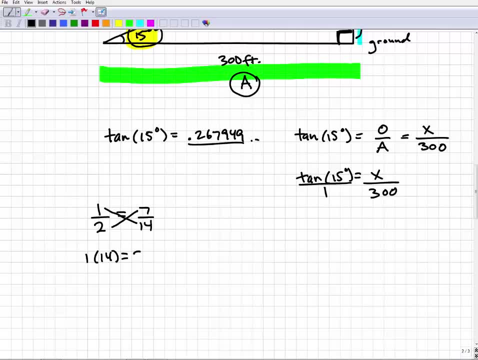 to be the same as if we multiply across this way 2 times 7. so we could see 14 is equal to 2 times 7, or 14. okay, so when you have a proportion or two equal fractions, we can just simply cross multiply, okay. well, it's called the cross product. that just means cross multiply and we can solve now, let's. 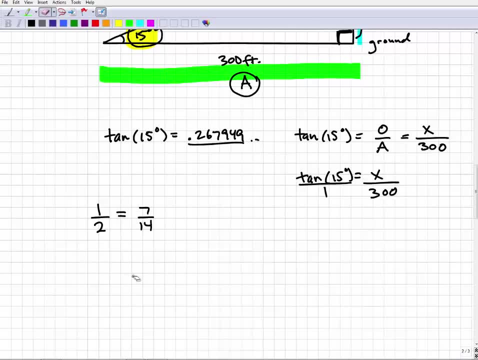 see how this works. okay, so let's suppose I have an equation. all right, let's get rid of that 7. let's put x. I have one fraction equaling to this other fraction over here, but I don't know what this value is. okay, well, let's cross multiply: 1 times 14 is 14, okay, and 2 times x is 2x. 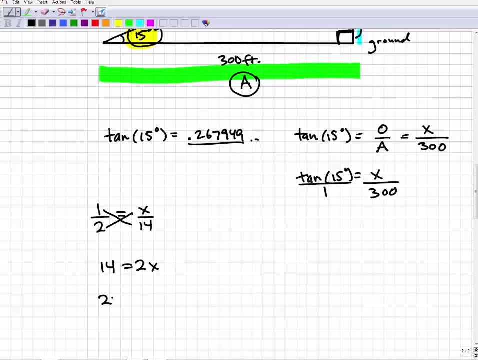 okay, so let's see how this works. okay, so let's suppose I have an equation. all right, let's get rid of this. so now I have this basic equation, let's write it this way: 2x equals 14, and I can solve for x. you have to course, know some basic algebra to be able to do trigonometry. so if 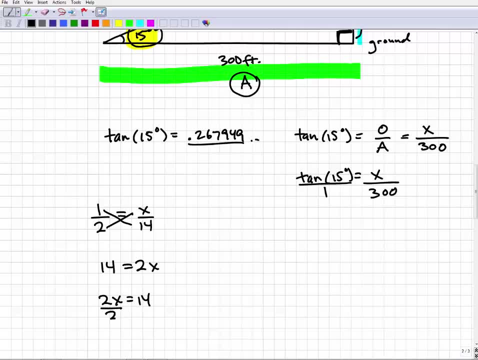 you're not. you don't know exactly how to do this. all we're going to do is just divide both sides by 2 and we get x is equal to 7, and that's the value right. this was 7. 7 over 14 is the same. 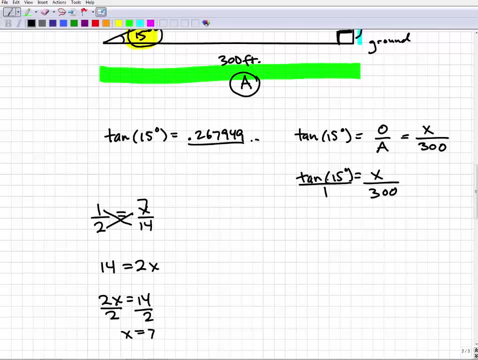 thing as one half. we're going to do the exact same thing here. okay, recognize this tangent: 15 degrees, the same thing as this decimal, and I can write any number over 1 when I want to create a fraction. in other words, 3 is the same thing as 3 over 1 as a fraction. if I want to look, 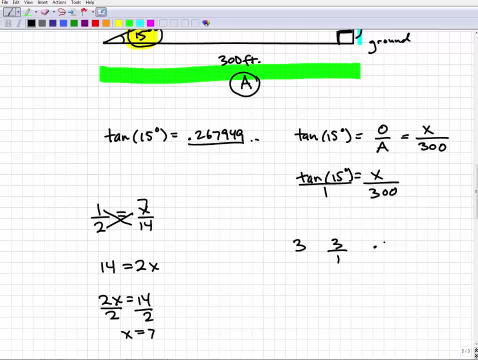 at 3 as a fraction, 3 over 1. if I want to think of 0.267 949 as a fraction, no problem, just take that thing, put it over 1, and now I have two equal fractions, because I know I can use this proportionally. 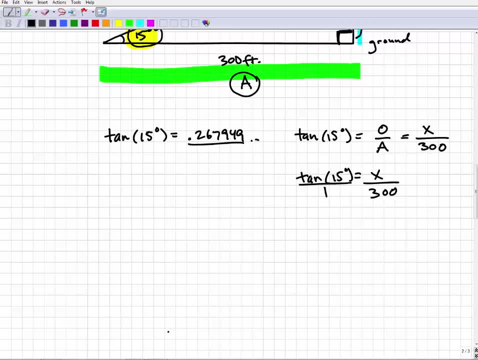 to solve this. okay, so let's go ahead and actually do this and we'll wrap this up. so we're going to multiply across, right, we're going to multiply these two together and then we're going to multiply these two together. all right, let's do this 1 times. X is simply just X, then tangent of 15 times 300. 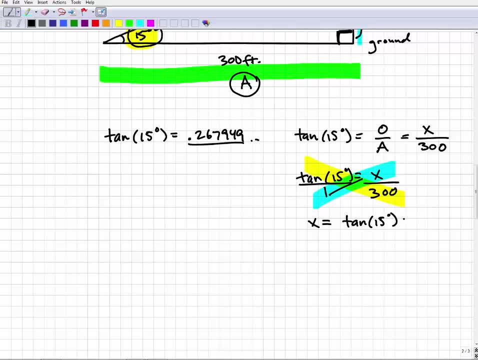 we'll write it this way: tangent of 15 degrees times 300. of course we know that the tangent of 15 degrees is the same as this decimal point: 2, 6, 7, 9, 4, 9, etc. you don't want to use in your. 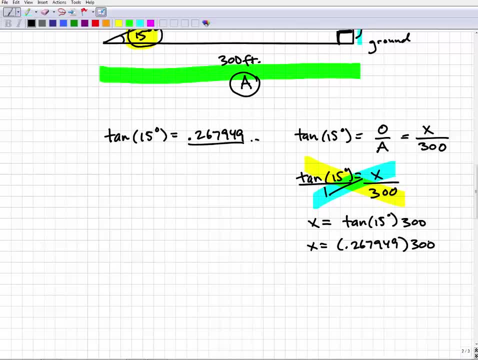 calculator, the full amount. we're going to multiply that by 300, okay, so let's go ahead and do that now and you can use whatever available device you have. if you have a calculator, that'll be great, or you can use your like online calculator. of course you don't want to do this by hand, you can just follow. 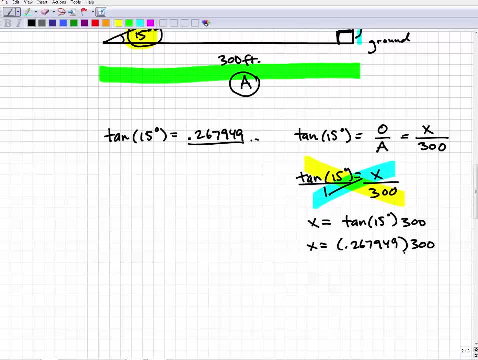 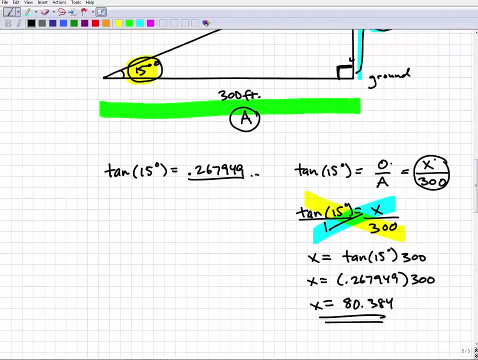 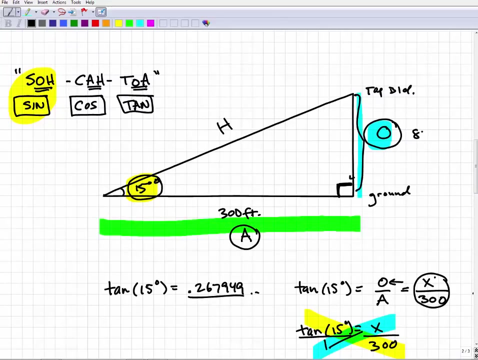 what I'm doing, but answer roughly. when we do this, multiplication is going to be somewhere around 80.384.. Okay, and that's our answer. Okay, x, remember, when we set up, this fraction is the same as the opposite, so that means our building over here, or whatever distances this is, was 80.34 feet, 80.34 feet high, and that's. 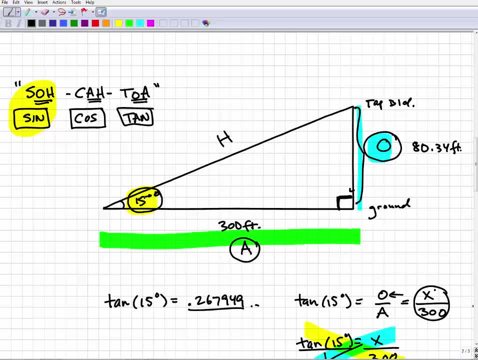 it. Okay now, of course. I mean I gave you the explanation, but if you were able to get the degrees here and get this measurement and this, you can get very precise right. you can measure, you can walk this out, you can do all kinds of ways and you can get the measurement of angles. 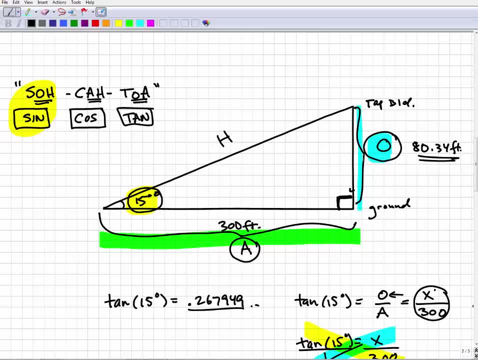 very precise as well. and here we have the exact, precise distance of this side of this right triangle, and it's very easy from this point to get the distance from here to here. So this is the fundamentals of trigonometry. it's everything is built upon. 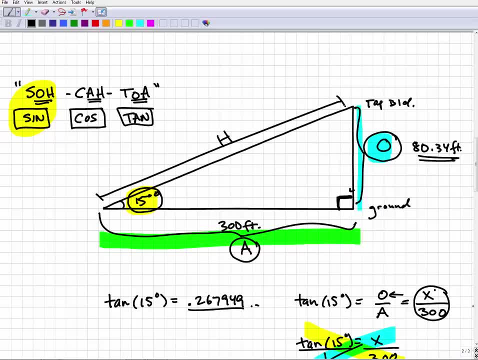 this right triangle. trigonometry In trigonometry, the applications are just amazing. Okay, in a former life, before I was a, before I taught mathematics, I was in the military. I was also in the Marine Corps. I was also a Navy officer. One of my tours as a Navy officer is I served as